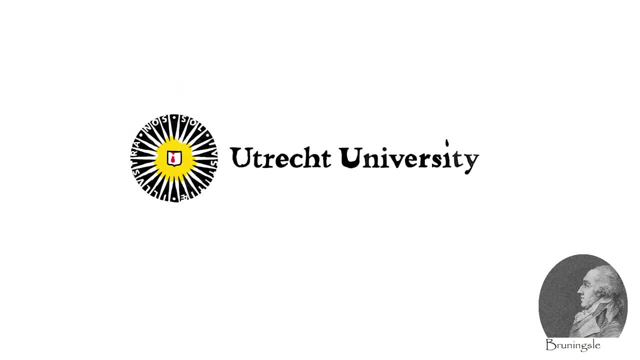 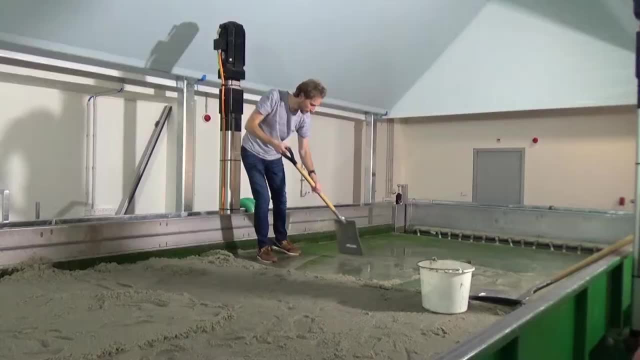 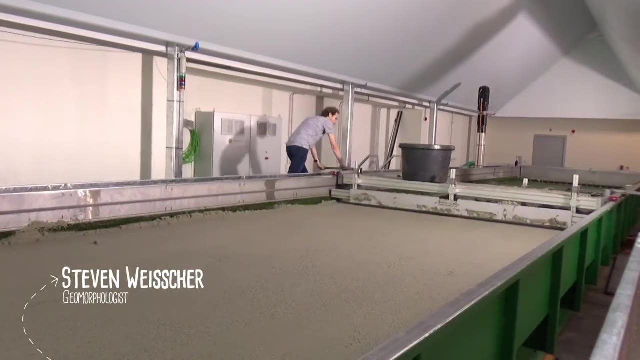 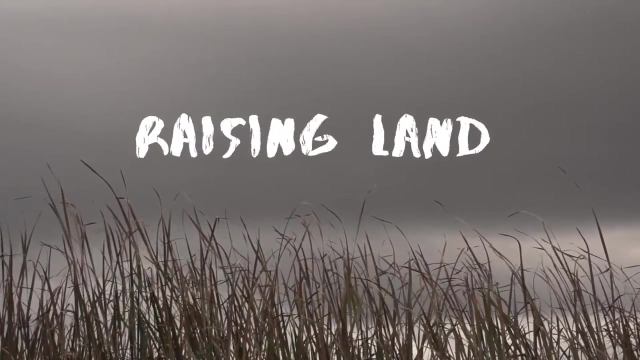 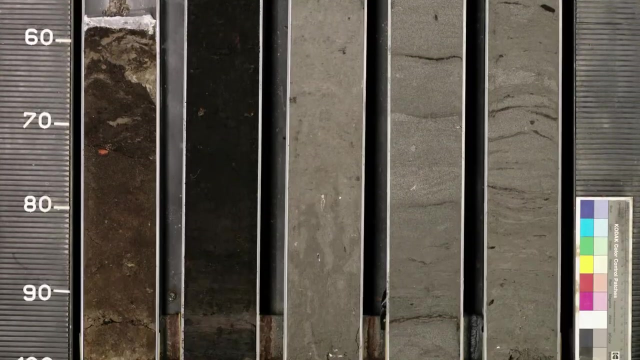 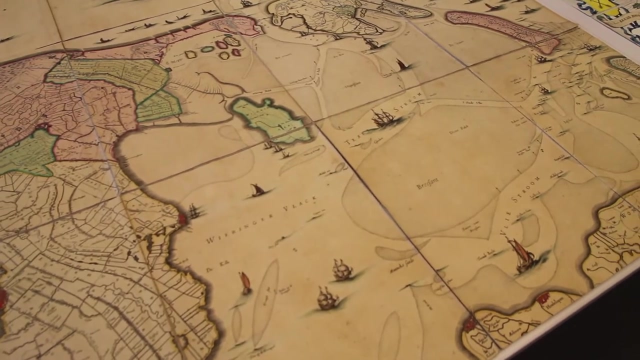 My name is Steven Weijsje and I study how estuaries build and raise land. Geological records in the form of boreholes and old maps show us that many old estuaries were able to form new land and keep up with mild sea level rise. 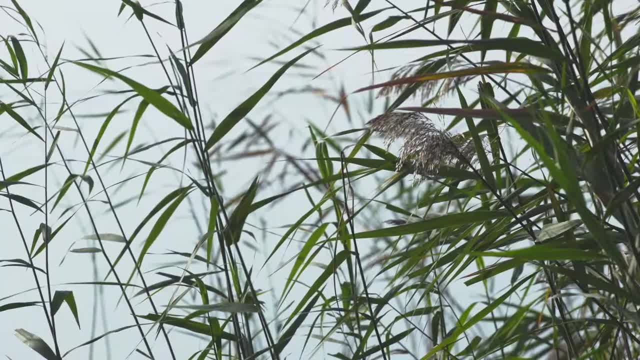 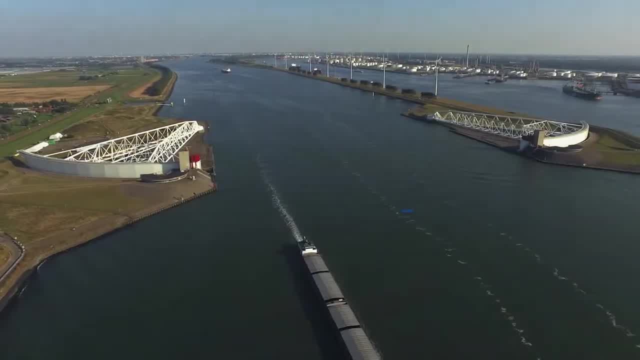 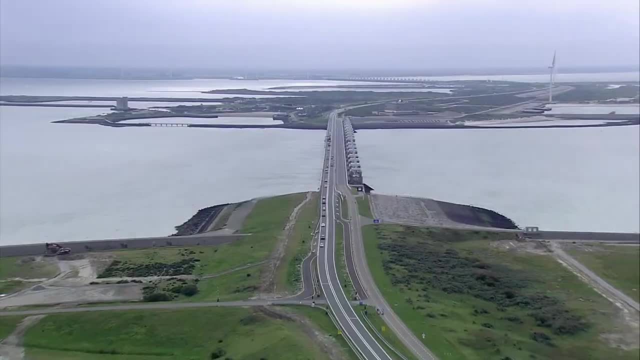 In turn, this valuable land opened up new opportunities for plants, animals, agriculture and urbanization. However, most present-day estuaries are engineered, dredged and bounded by dikes and are therefore not able to keep up with sea level rise. 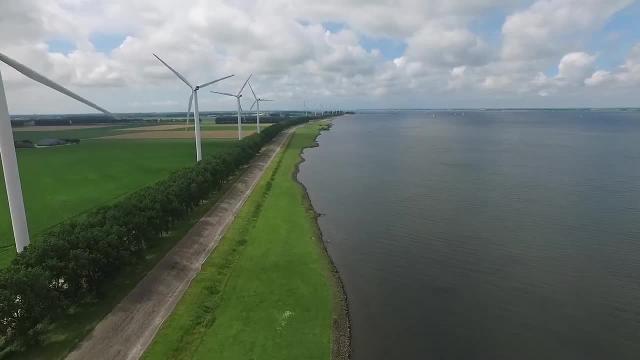 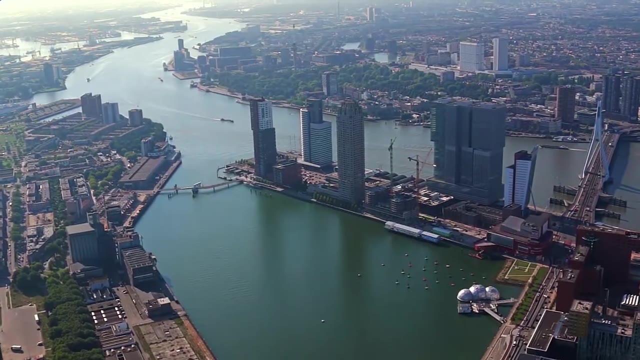 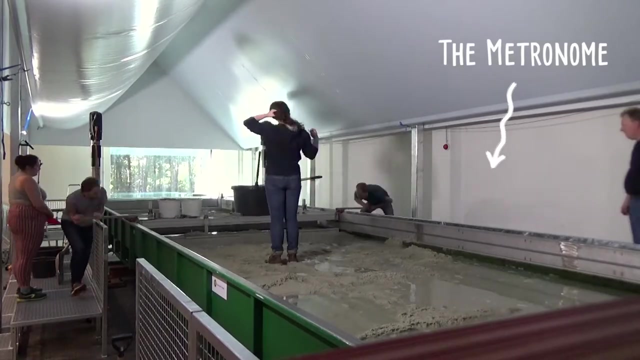 We need to understand which processes are important to build and raise new land in and around estuaries which will contribute to natural solutions to let our coastal regions grow with future sea level rise. To solve this, I use scale experiments through which I study the development of infilling. 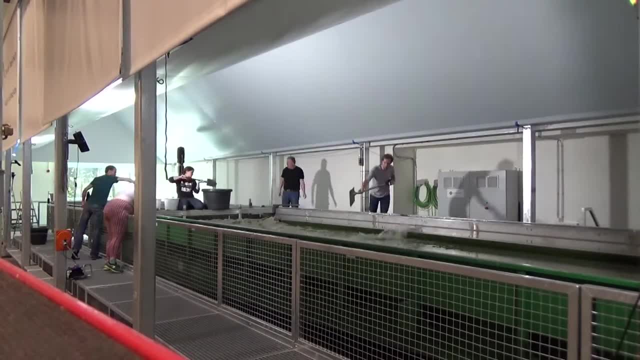 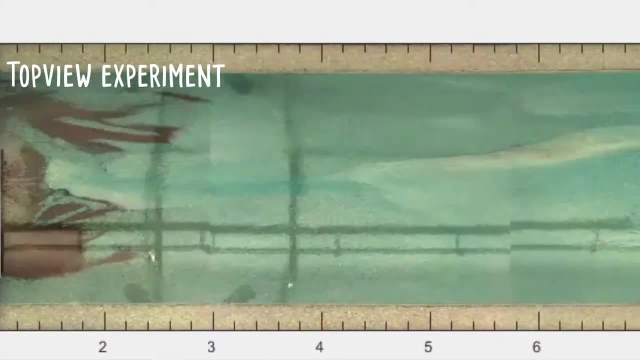 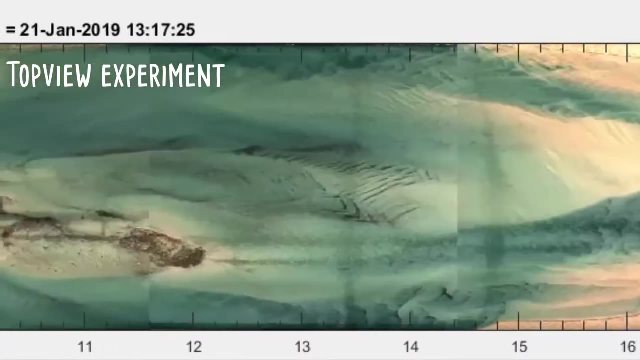 estuaries. I ran scenarios with mud and live vegetation and computed flow in the flume using a computer model. My research shows that mud and especially vegetation help bars to grow above the high tide water level and stimulate infilling from the river towards the sea. 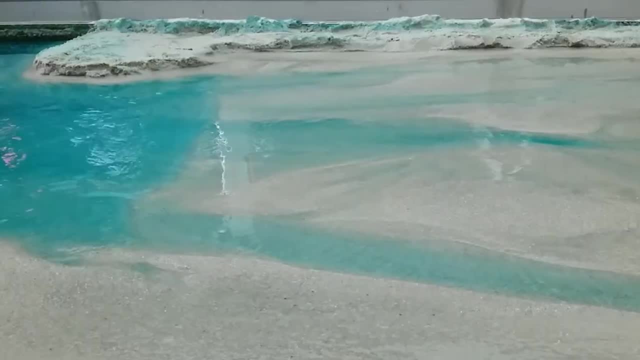 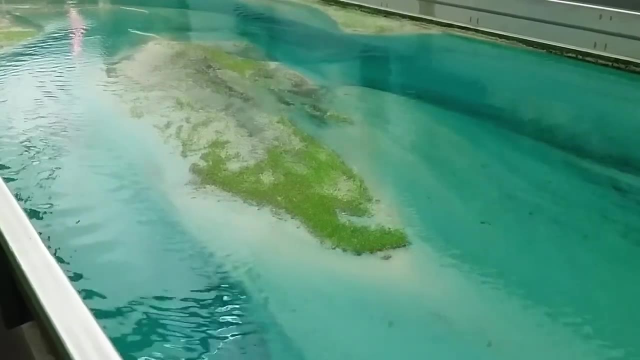 This narrows the estuary and reduces the amount of water that flows in and out of the estuary. In addition, vegetated bars and lands are more difficult to erode than muddy bars. It is mainly vegetation that fixates bars and reduces the migration of channels. 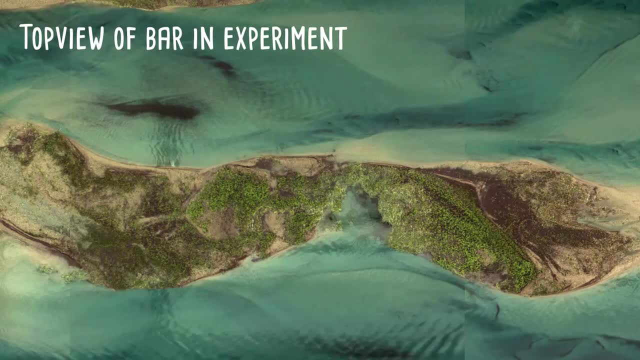 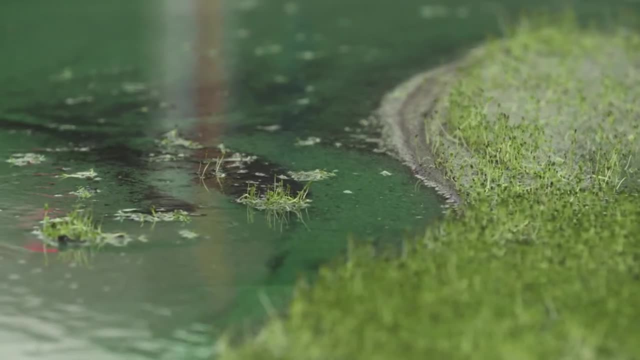 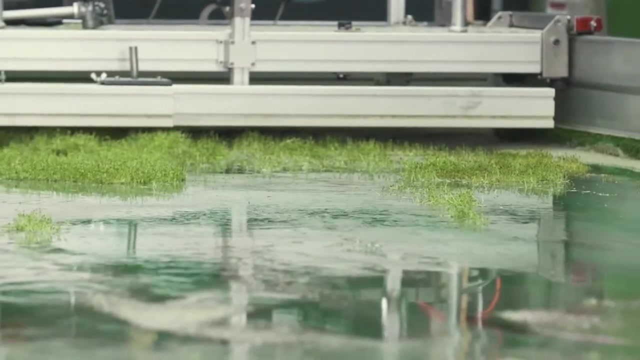 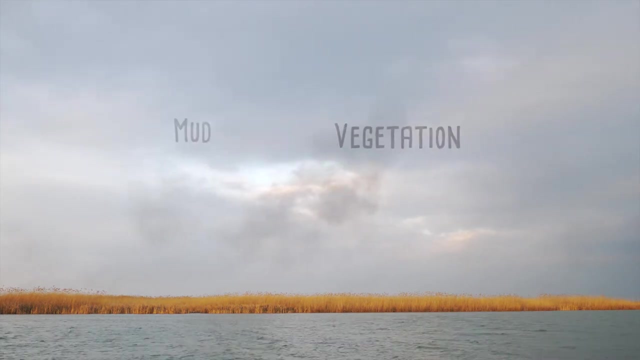 This effectively extends the lifespan of newly formed plants. In light of the rising sea level, these experiments have brought us one step closer to developing natural solutions to protect our coastal regions from drowning by building and raising new land with mud and vegetation. This will contribute to more resilient delta estuaries for future generations. 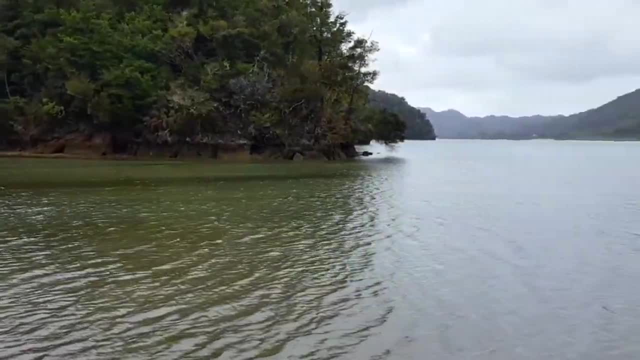